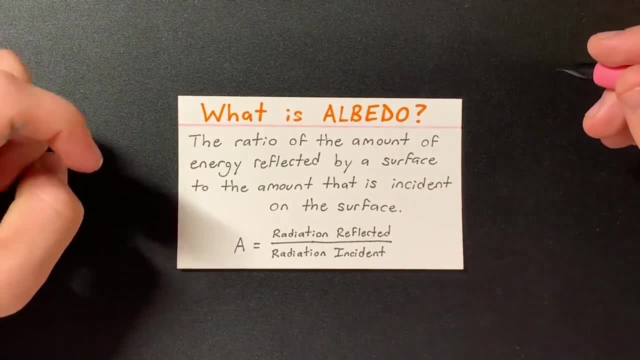 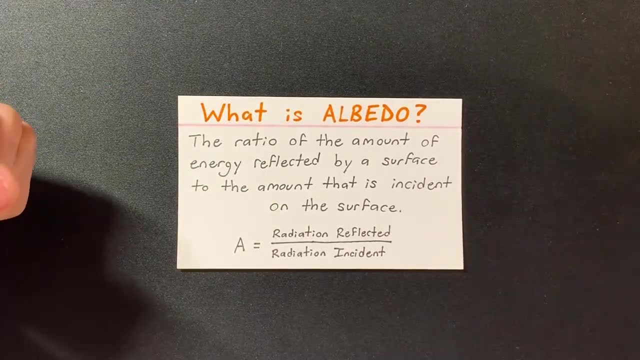 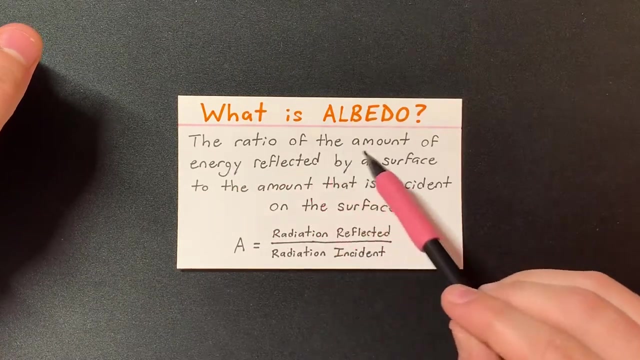 Hey, what's going on everybody? Welcome back to Earth Science Ed. In today's video I will be discussing albedo, in terms of meteorology really. So the question is, what is albedo? And basically the scientific definition is the ratio of the amount of energy. 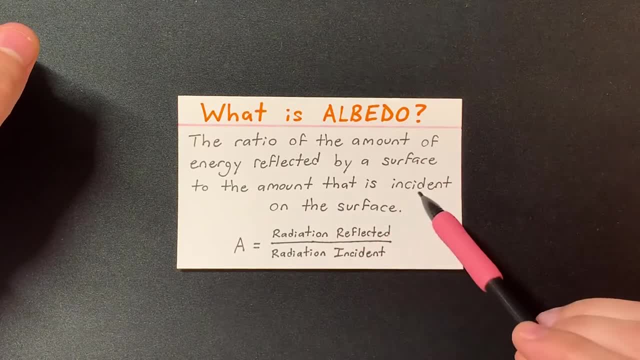 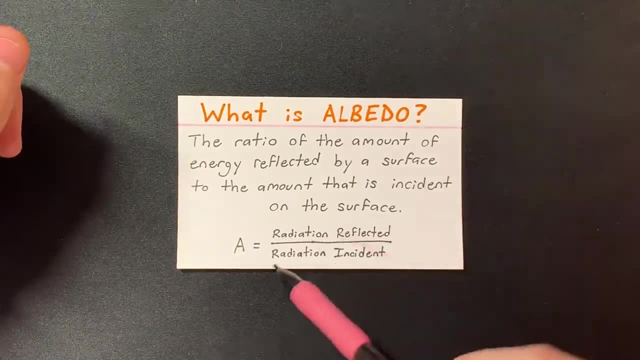 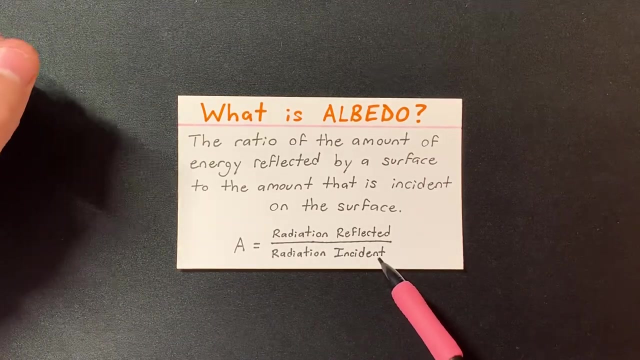 reflected by a surface, to the amount that is incident on the surface. So this is a little bit of a confusing definition, but to put it in mathematical terms, the albedo is going to be equal to the radiation reflected divided by the radiation, the incident radiation right. So 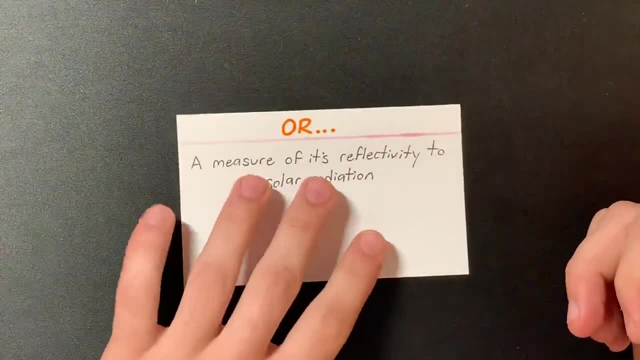 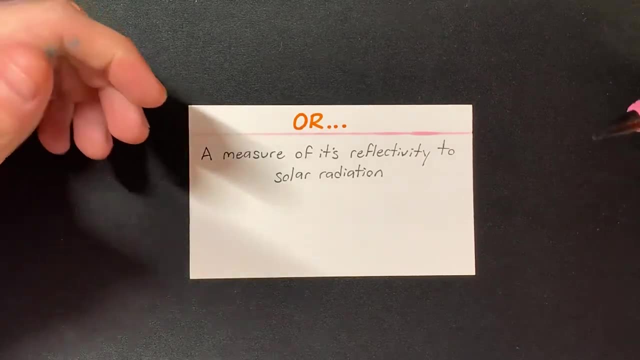 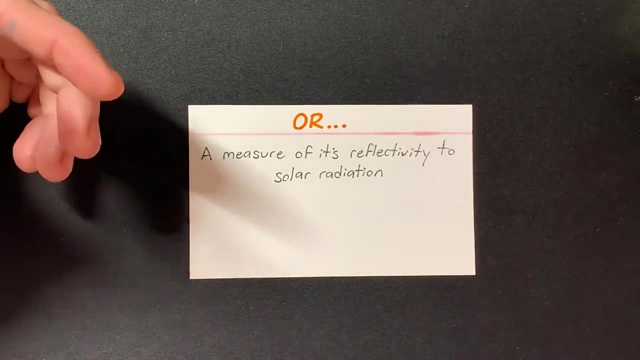 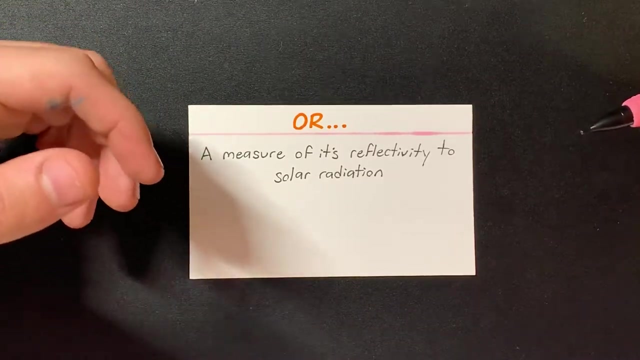 to make it a more simplistic definition, it's basically a measure of its reflectivity to solar radiation, right? So, like I said, we talk about albedo in terms of solar radiation a lot because of the reflectivity of certain materials, snow, dirt, just stuff like that. Obviously we know that. 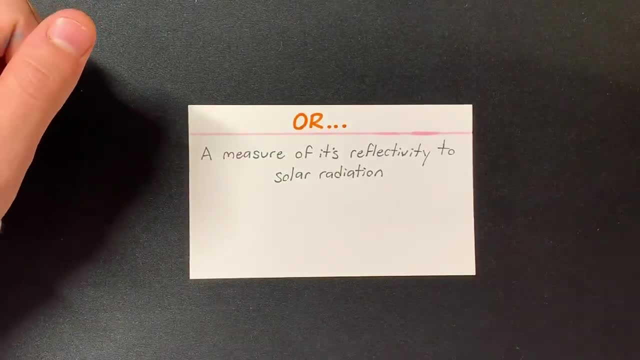 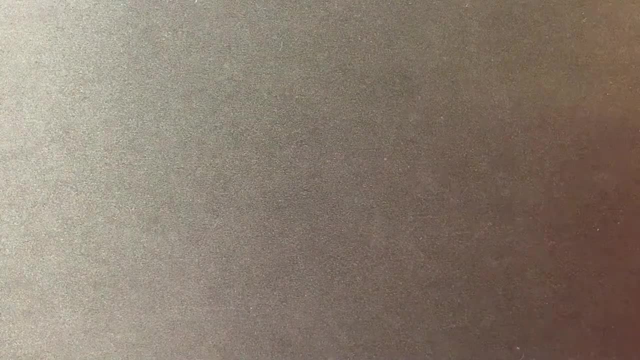 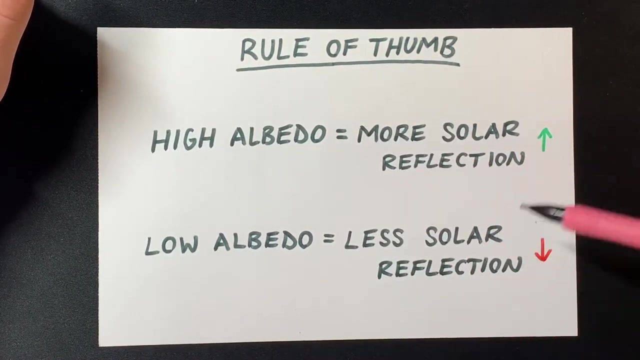 snow is going to have a higher reflectivity right And basically I'm going to explain why that is the case. So a good rule of thumb for albedo is that the higher the albedo, the more solar reflection, and the lower the albedo, the less. 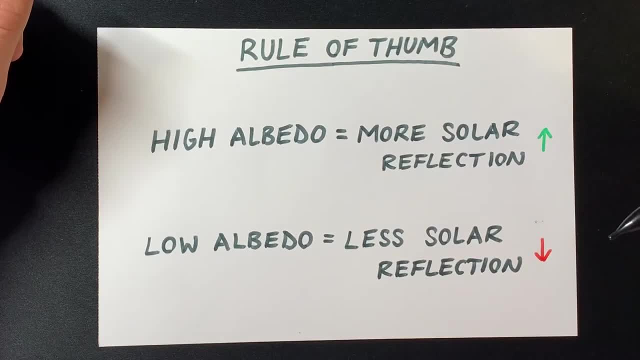 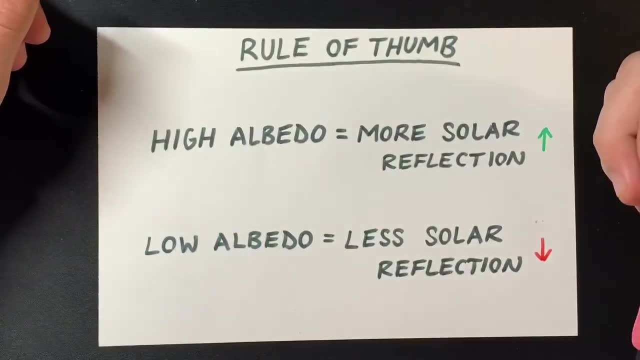 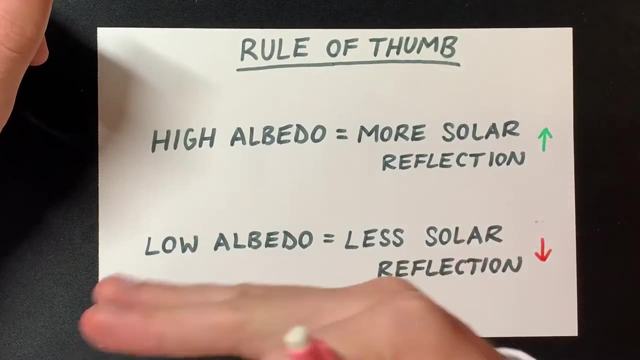 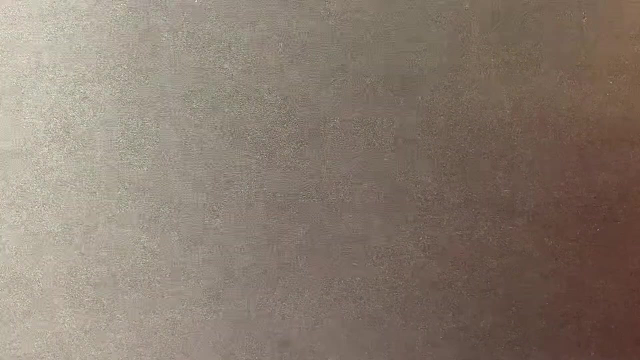 right. Pretty easy to memorize, right? So, basically, the higher the albedo, the more reflection will be caused on a surface, and the lower the albedo, the less reflected solar radiation of that light, right? So here I wrote down some typical albedo values that are in everyday life. 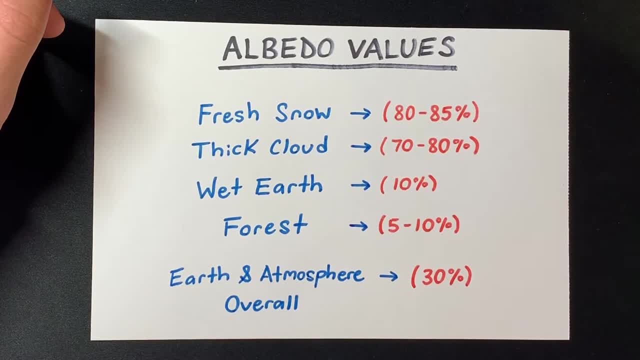 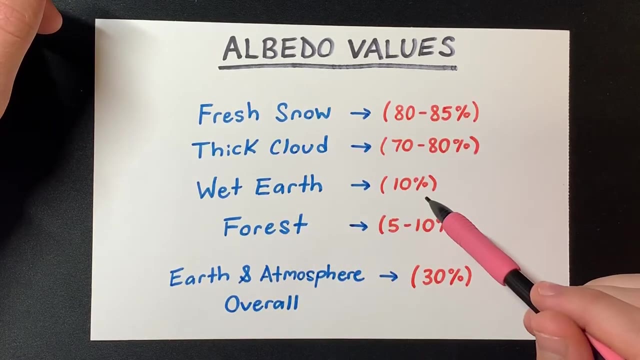 right, So fresh snow is going to have a very high albedo at 80 to 85%. right, A thick cloud is going to be 70 to 80% And once we drop to the darker surfaces like wet earth, that is all the way down at 10%. so a very low albedo, right. So not much light that hits.